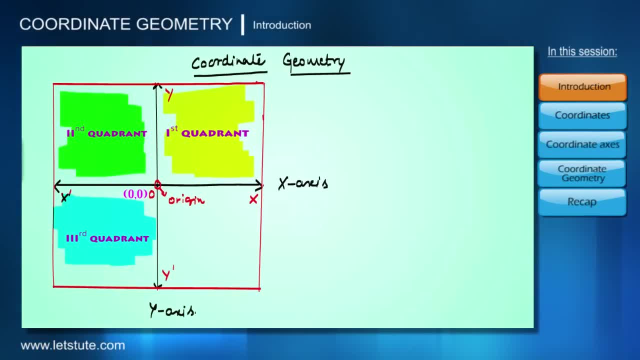 called as first quadrant, second quadrant, third quadrant and this is fourth quadrant. And the x-axis possess positive values on the right side of the origin and it possess the origin. Similarly, y-axis possess positive values above the origin and it possess negative values below the origin. And these values of x and y-axis help us to find the location. 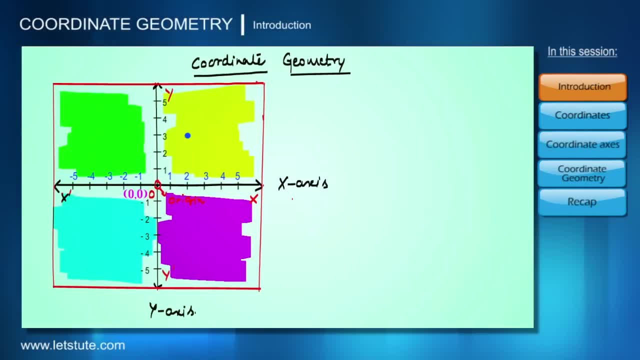 of any point on the plane, For example. here is the point. I want the location of this point And for finding the location we require reference. So we will take reference of x-axis and y-axis, So we can see that this point is covering. 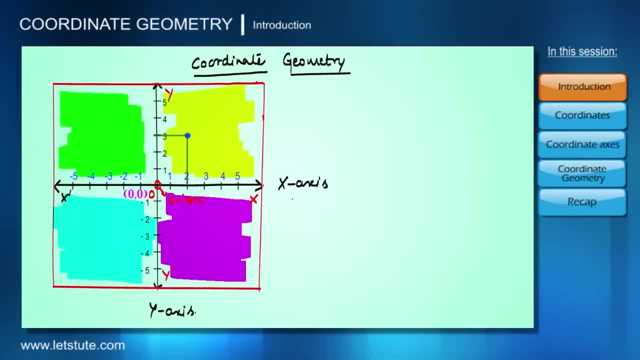 two units. It is 3 units on positive x-axis and 3 units on positive y-axis. So therefore its location will be given accordingly: 2 units for x-axis, 3 units for y-axis. This kind of representation of the location of a point is called as coordinates, And the value of x-axis is called as x-coordinate. 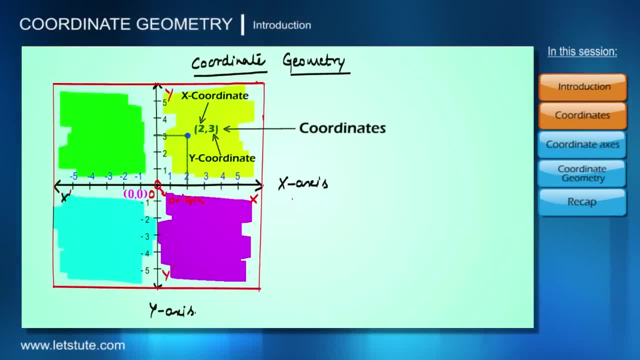 and the value of y-axis is called as y-coordinate, X-coordinate is also called as abscissa and y-coordinate is also called as ordinate. about the coordinates, we can say it is a location of a point, or in other words, we can say it: 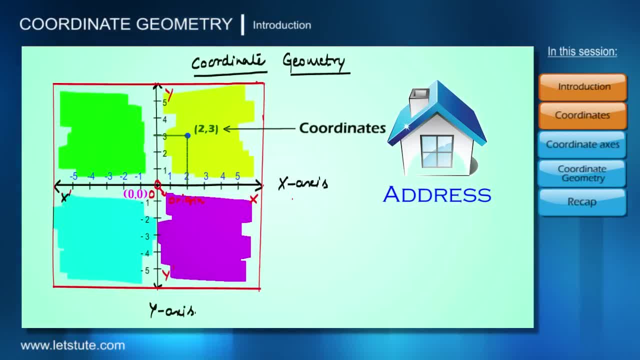 is address of the point. For example, if I want to write address of my home, I will give the street number, the lane number, the area code, etc. All these things are references to reach my home. Similarly, these coordinates are the references for locating a point on. 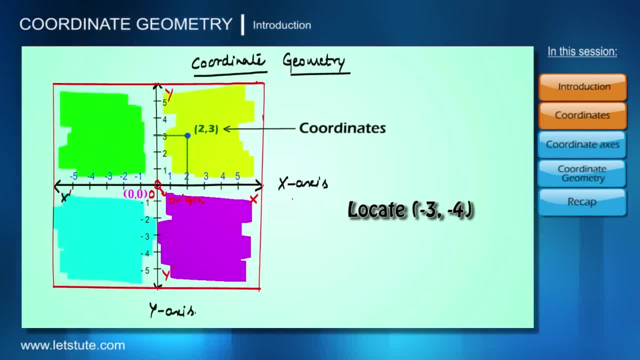 the plane. Suppose we are given with the coordinates and we want to locate this point. So we will first take the x coordinate, that is minus 3, and x value is minus 4, that is y coordinate. Now we can see that they both are intersecting at this value. So this: 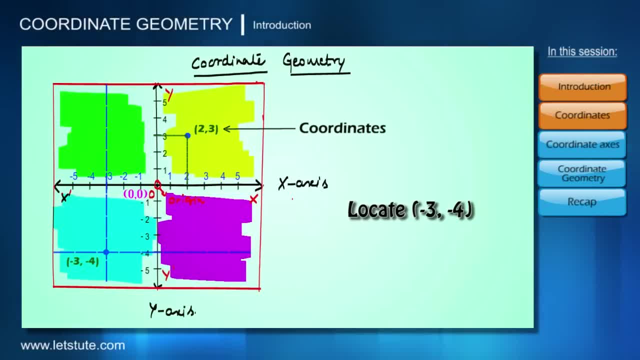 is nothing but minus 3 comma, minus 4.. So this is how coordinates work. Now let's talk about the sign of the coordinates. It depends on the quadrant in which they exist, And these two reference axes, x axis and y axis, are coordinates. So these two reference axes, x axis and y axis, are coordinates. So these two reference axes, x axis and y axis, are.